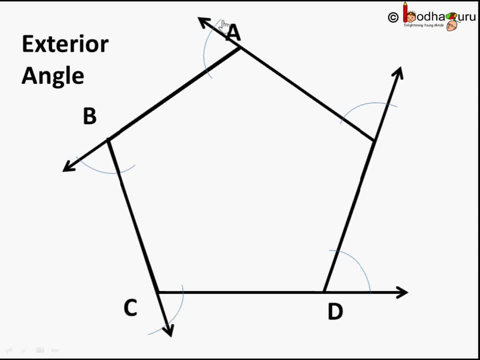 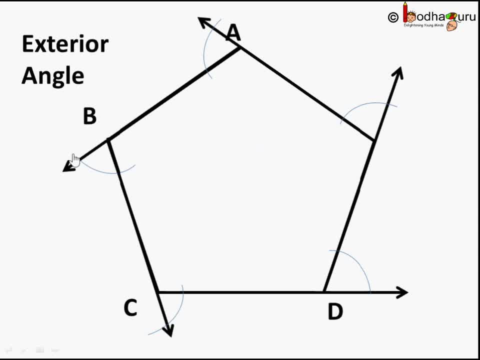 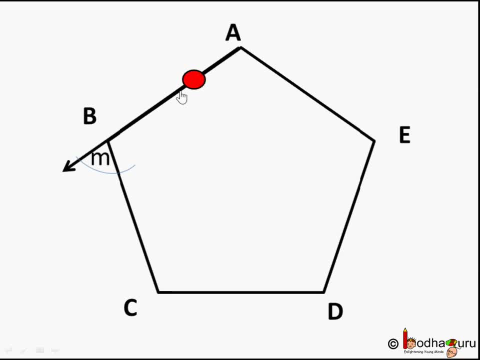 come back to this point while walking on the boundary. So I start from this point, keep walking. As soon as I hit this point, I need to turn. I need to turn left. if I'm walking this direction, I'm going to turn left to start walking this. 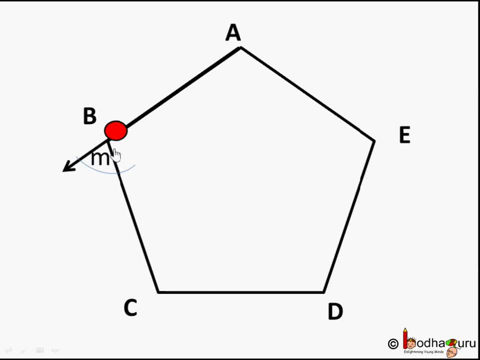 side. So I turn by an angle M And then I start walking here. Then as soon as I reach this point, I again turn by an angle n- this is the exterior angle- And I start walking here, walking on this side. then as soon as i reach this point, i need to turn again to walk on this line. 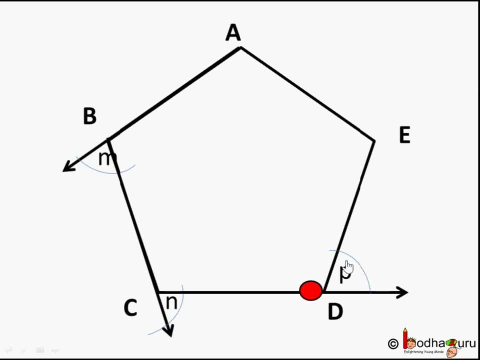 i need to walk on the boundary right, so i turn by angle p and i start walking on this side, this boundary of this pentagon shaped park, and i, as soon as i reach point e, i need to again turn by an angle exterior, angle q, to start walking this way, and then, when i reach point a, i again. 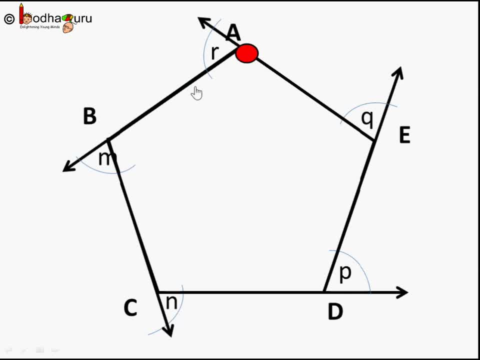 turn by an exterior angle r to start walking here till i reach my starting point where i started. so i walked on the boundary of this pentagon and, as you can see, i turned five times by an exterior angle m here to start working here. by an angle n to walk on this side. by an angle p to 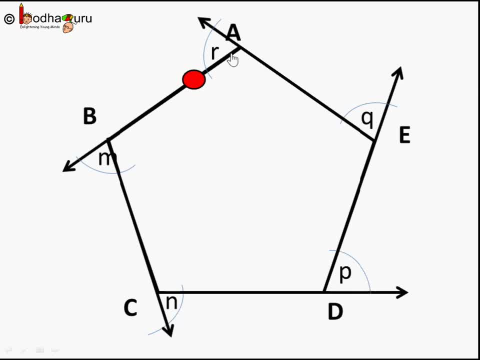 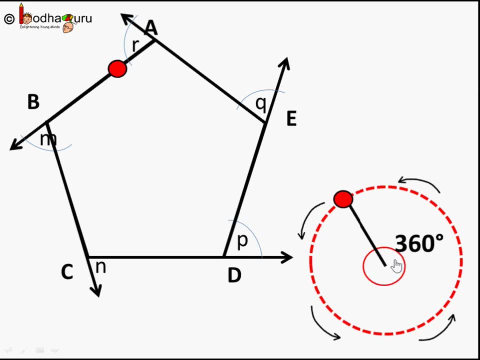 walk on this side, by an angle q to walk on this side and by an angle r to come till here. and if you observe carefully, this is very Speedlike, similar to: if suppose you are walking on a circular path. right, you are going to really go.